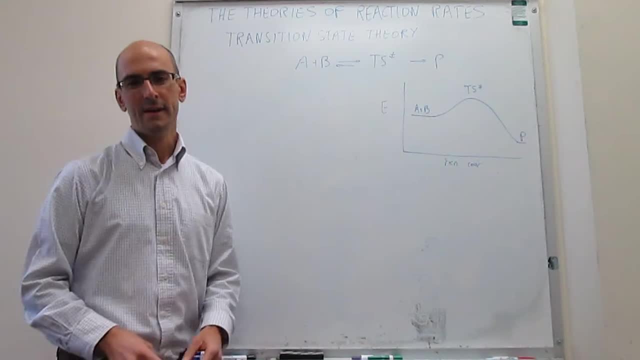 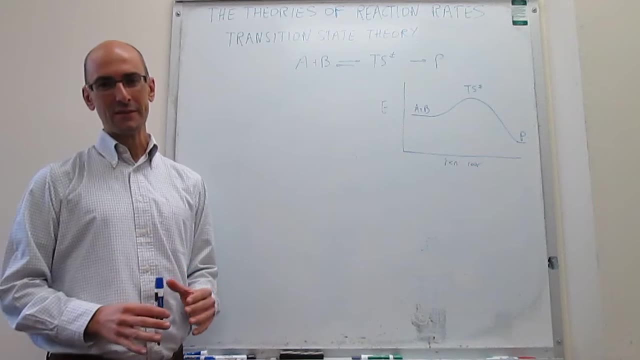 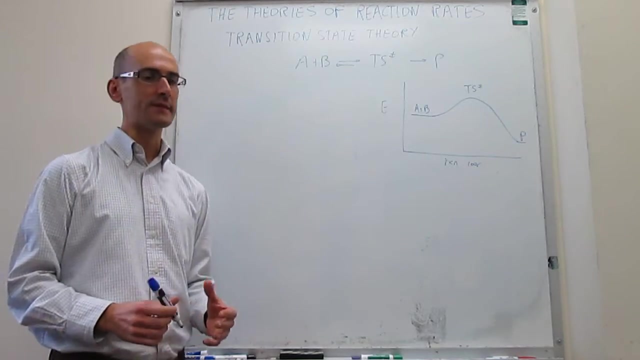 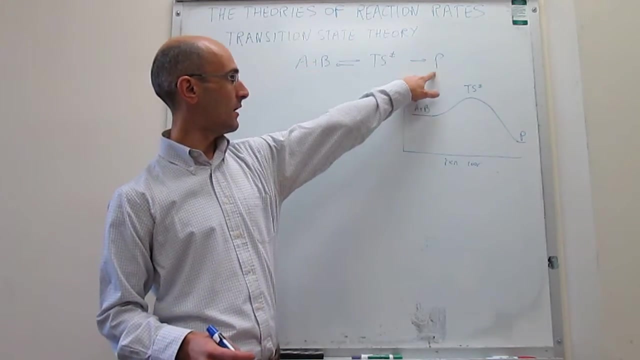 In this video we describe transition state theory from a thermodynamics formulation. So transition state theory is one of the most successful techniques to calculate rate constants without ever having to do an experiment. The gist of the theory is that you can write a reaction in which two radians, A and B, come together to unite products as having this. 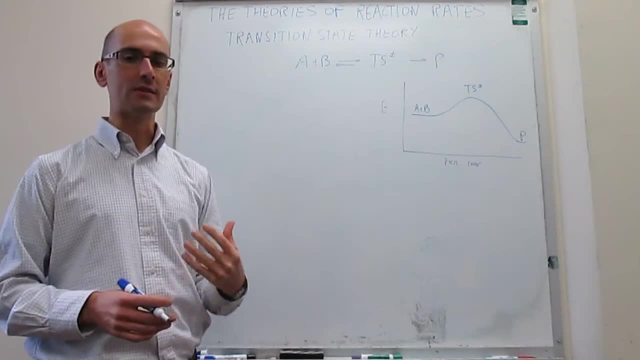 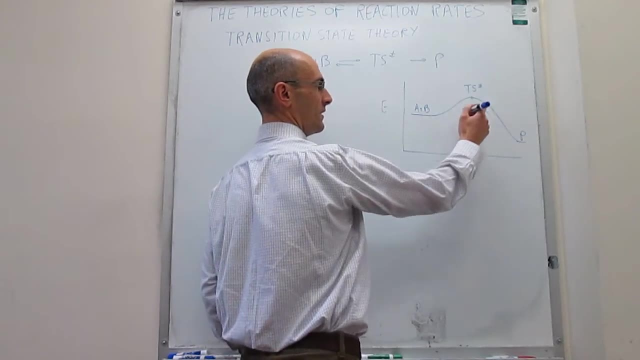 reaction scheme in which this intermediate would be a transition state. Now, the transition state is not a stable intermediate. Instead, it's simply the point of maximum energy along the minimum energy reaction path connecting radians and products. Now, in a prior video, 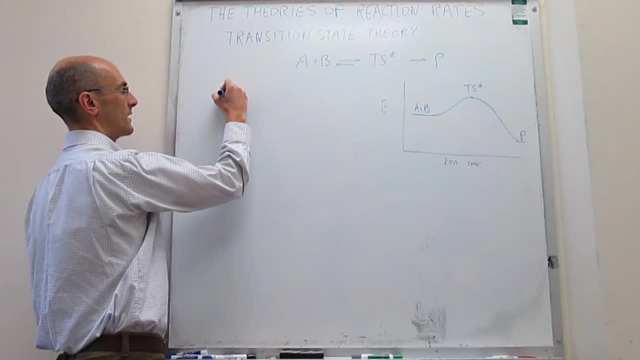 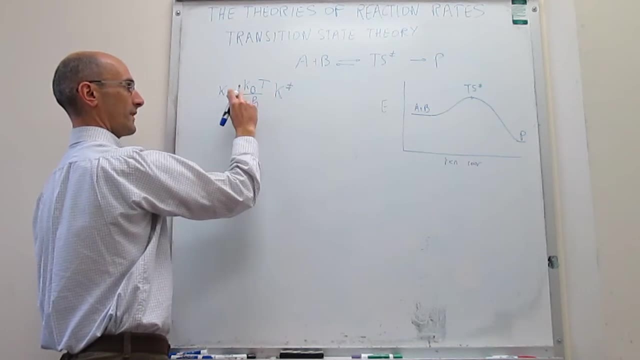 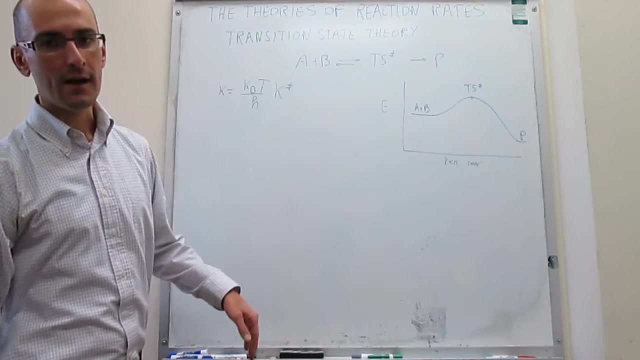 we have seen how the theory essentially tells you that the rate constant for that reaction can be simply calculated as this: OK, well, that's Boltzmann constant, That's flux constant, That is the temperature, And then we have that this will be the equilibrium constant that gratifies the equilibrium between: 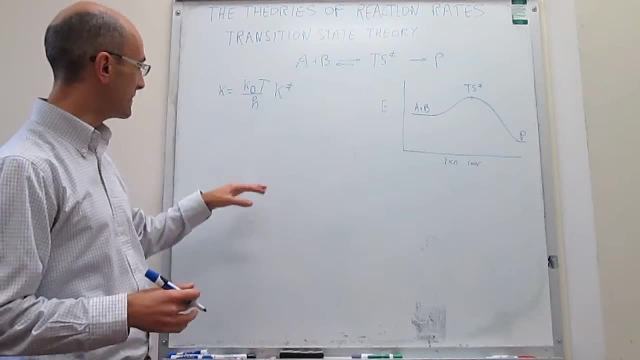 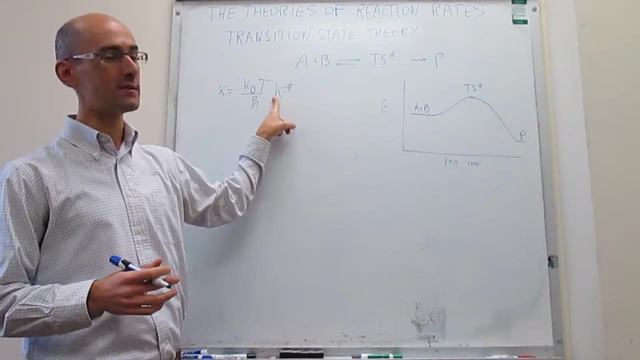 radians and the transition state. In this video we actually take this concept a little forward, And then we're going to try to see how we can use thermodynamic arguments to learn more about that equilibrium constant And, in the end, be able to explain things. 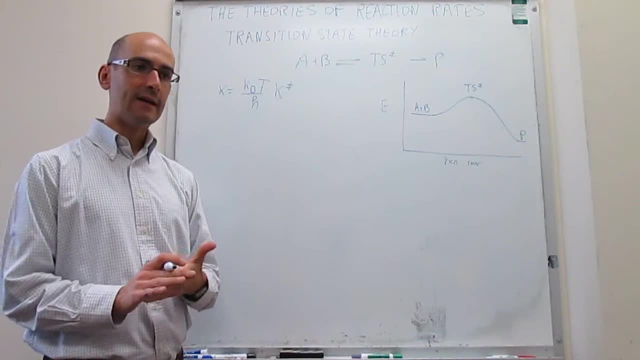 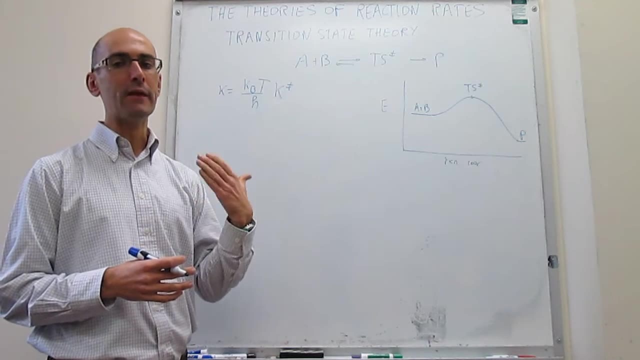 like the pre-exponential factor and the activation energy that are part of the Arrhenius theory. OK, in terms of changes like things like the Elflopi of activation, the Gibbs energy of activation and the Andropi of activation. 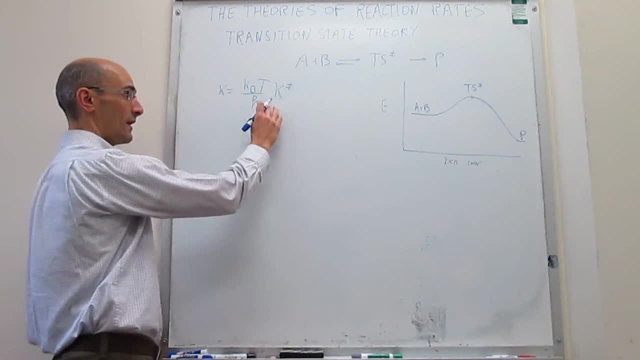 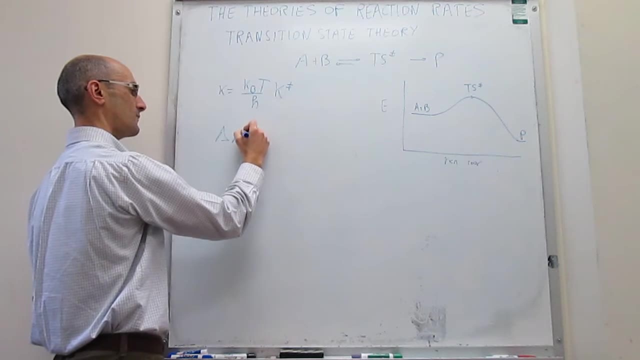 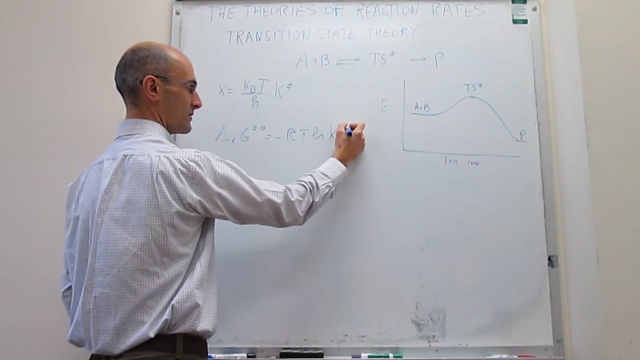 All right. so for thermodynamics, we know that equilibrium constants are related to the standard Gibbs energy. OK, so we know that this expression is one of the most important ones in all of thermodynamics. OK, that's the relationship between the equilibrium constant. 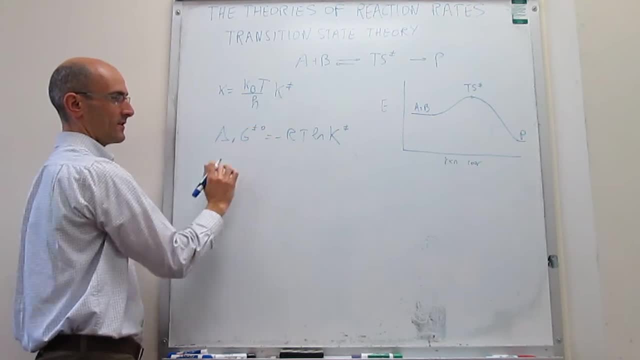 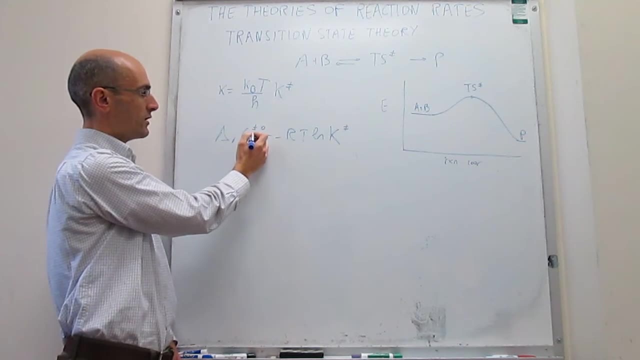 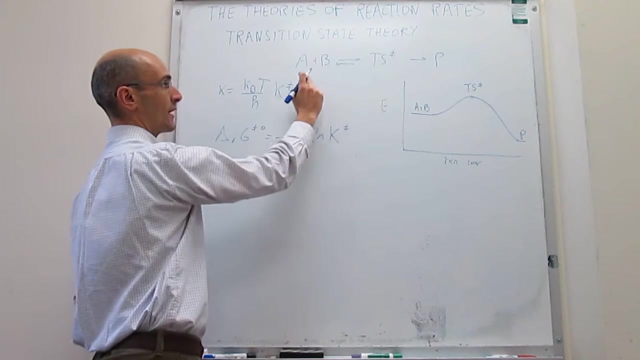 of a process and the Gibbs energy of the standard state. The other modification that we're actually taking here in this expression is that now this will be the Gibbs energy of activation, And that is the equilibrium constant that is responsible for the equilibrium between radians and the transition state. So the Gibbs 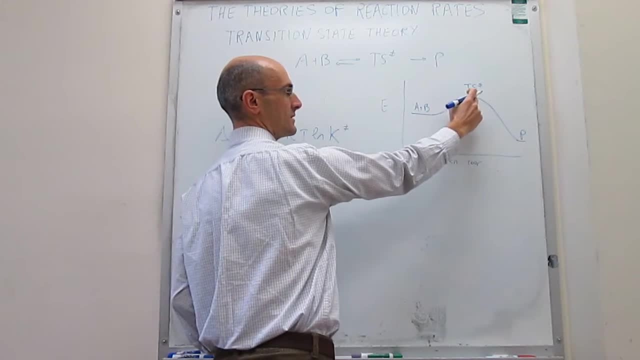 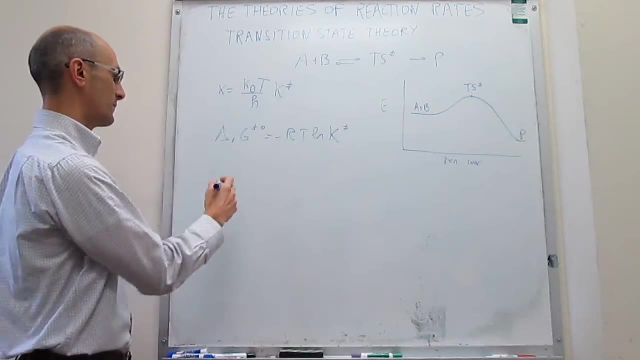 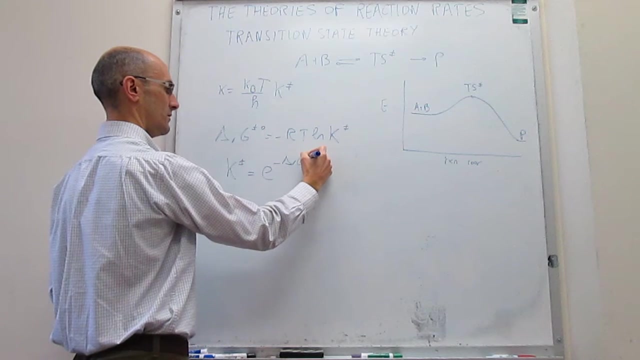 energy of activation will be the difference in Gibbs energy between the transition state and reagents. That will be delta G of activation under standard conditions. OK, so from here we can actually take and solve for the equilibrium constant, which is simply going to be e to the minus delta RG, not of activation over RT. Right And with 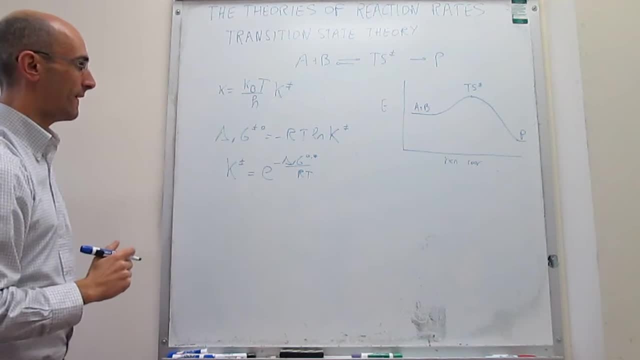 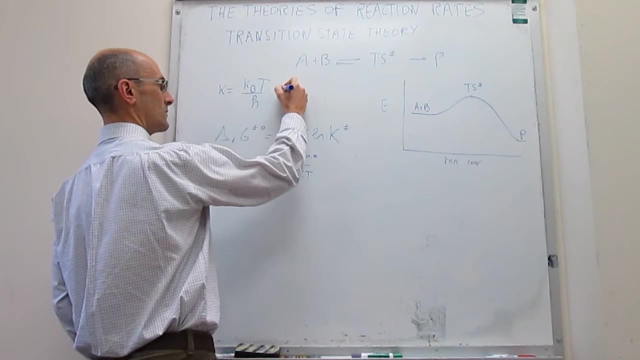 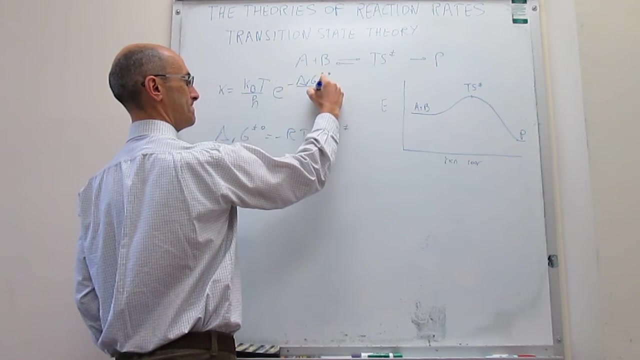 this value of the equilibrium constant, then we can come here and then find a new expression. All right, so that now is going to be using thermodynamic arguments. is going to be equal to e to the minus Gibbs energy of activation at the standard state over RT. Great, So that's. 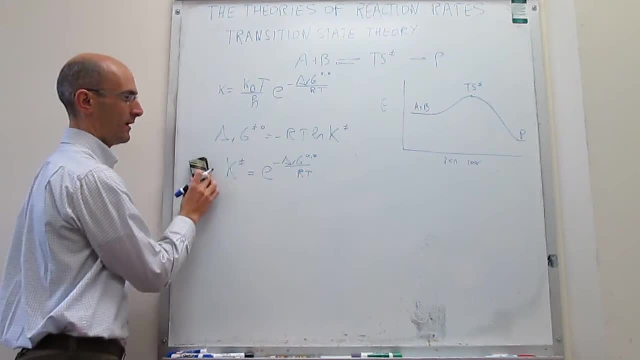 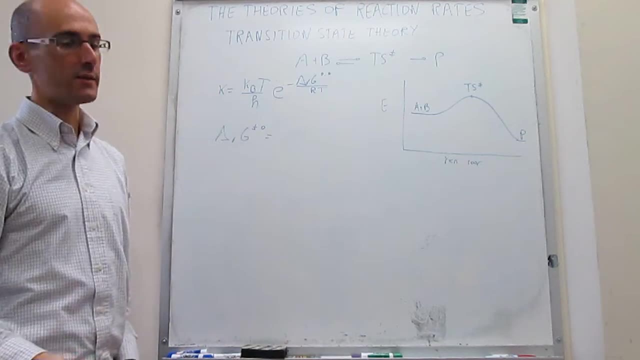 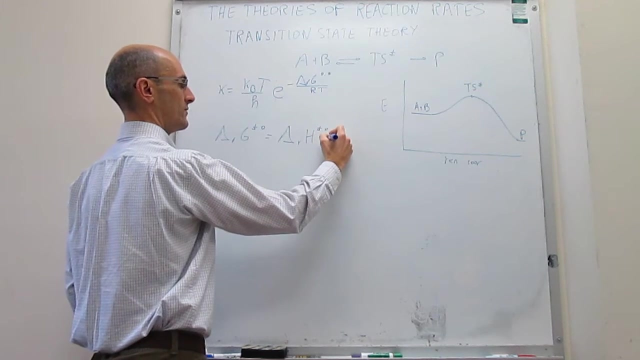 the first of thermodynamics that we include in our transition state theory. The second one is to recognize that the Gibbs energy is actually can be rewritten also as a function of the enthalpy of activation, the standard state and the entropy of activation of the standard. 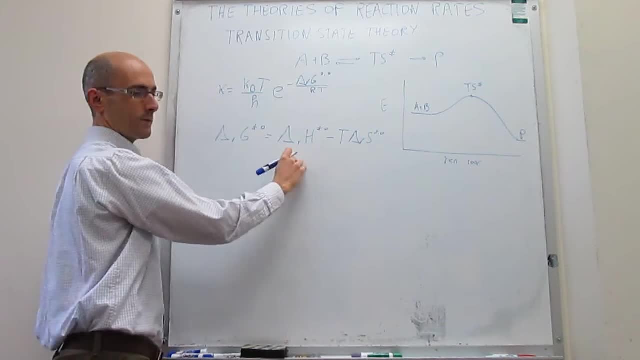 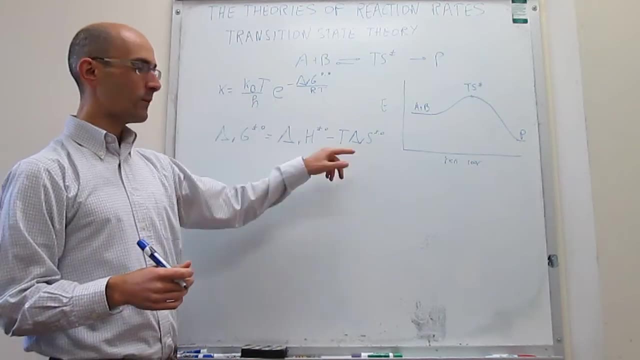 state OK Where this thing will be: the change in enthalpy as you go from reagents to the transition state. Again, that is what we call the enthalpy of activation, And it will be the change in entropy as you go from reagents to the transition state. 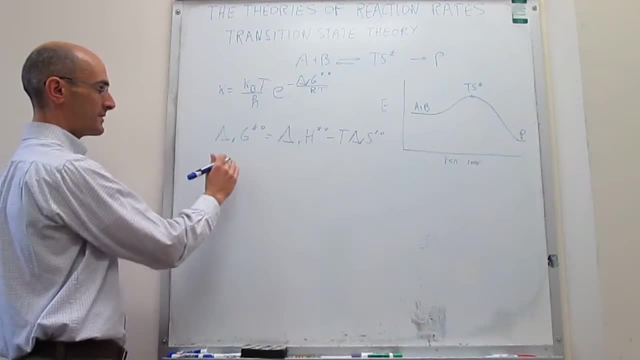 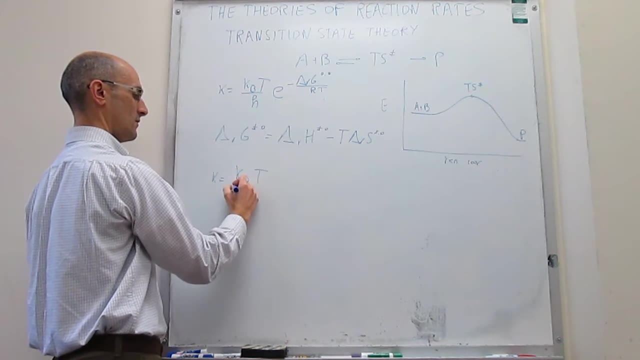 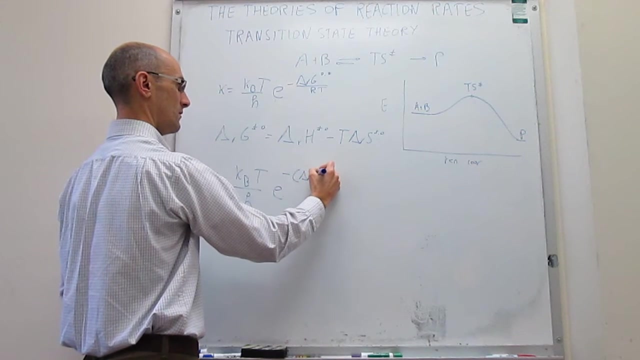 OK, so those are simple enough concepts, Right? so we can take this expression now and then replace it up here And we get that this is kB T over H, And then this will be e to the minus delta RH of activation minus T, delta RS of activation minus T. 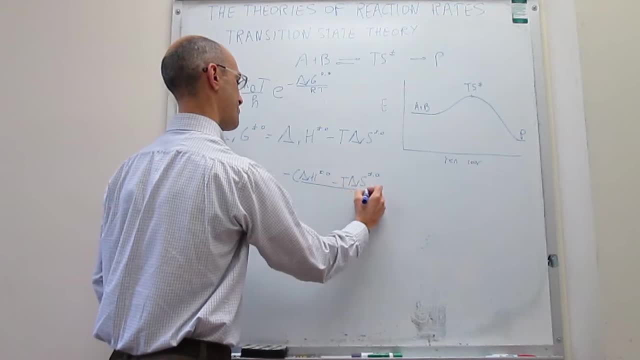 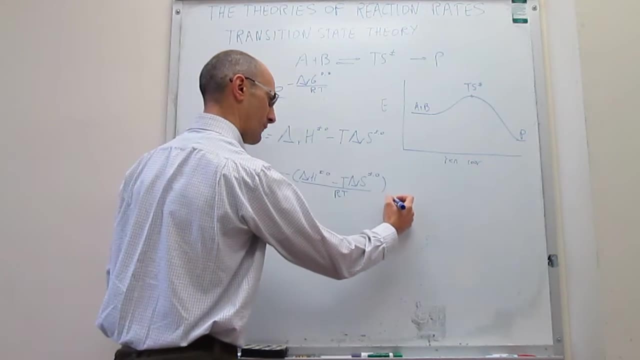 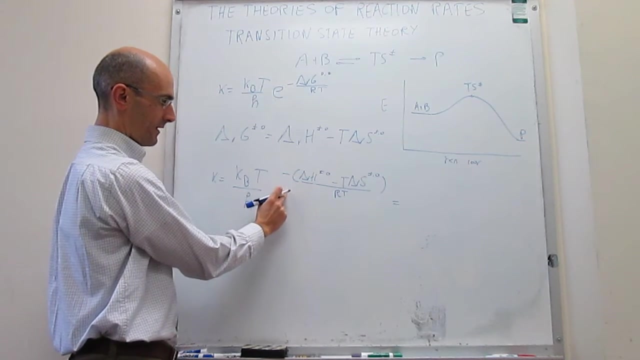 OK, OK, OK. So we have this is kB T over H over RT. OK, All right, So I'm folding that all forward. We're going to have two terms here: e to the minus, delta, RH over RT And then e plus. these things will cancel and it will be delta. 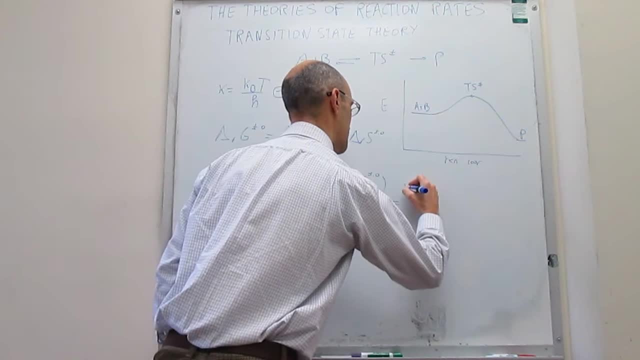 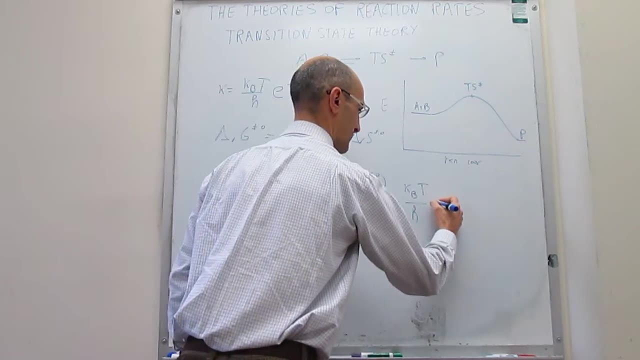 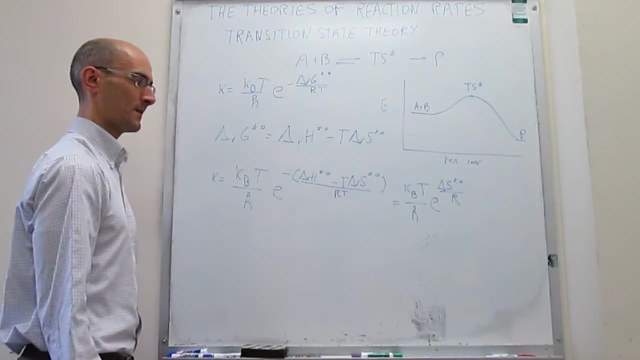 S over R. OK, so we can rewrite this as kB T over H. And then I'm going to write the entropy term first, which would be: e to the minus delta RH over RT, OK to the delta S of activation over R. and then there's the term that depends on. 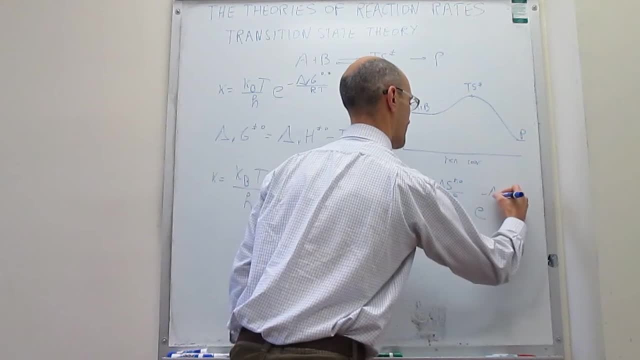 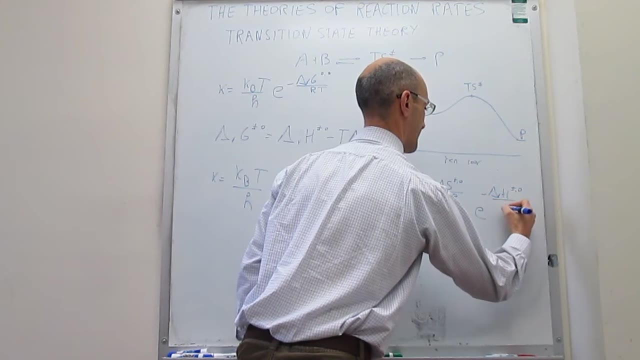 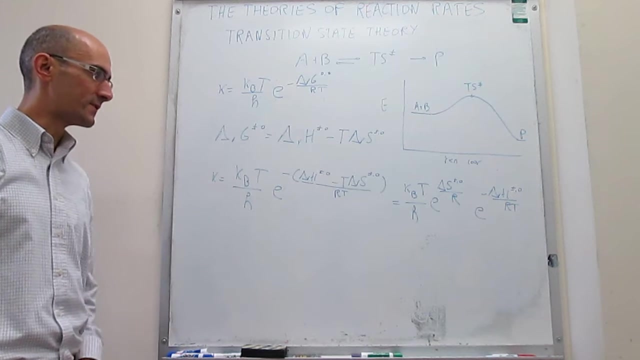 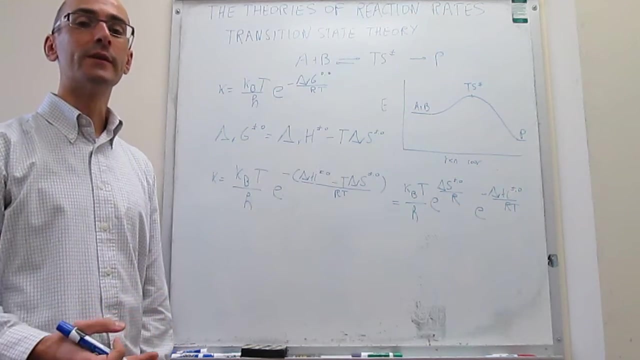 the enthalpy of activation minus delta Rh of activation over RT. okay, so this is now how we calculate our rate constant with transition state theory. now we can take a little pause here and then try to compare this to the Arrhenius expression. okay, notice that the Arrhenius expression would be: K is equal to A, e to the minus. 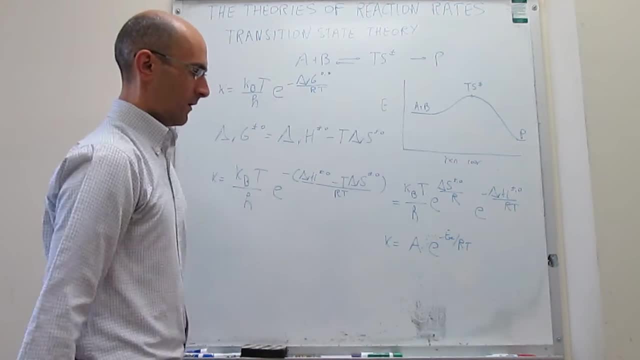 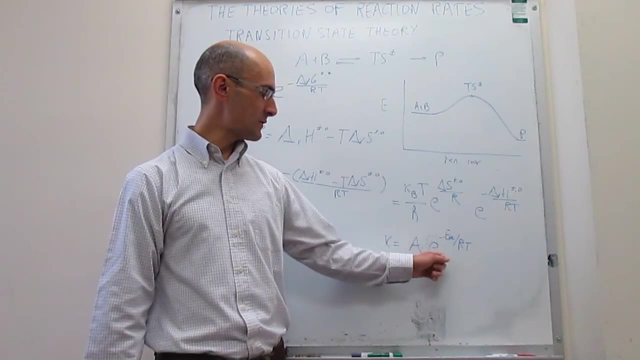 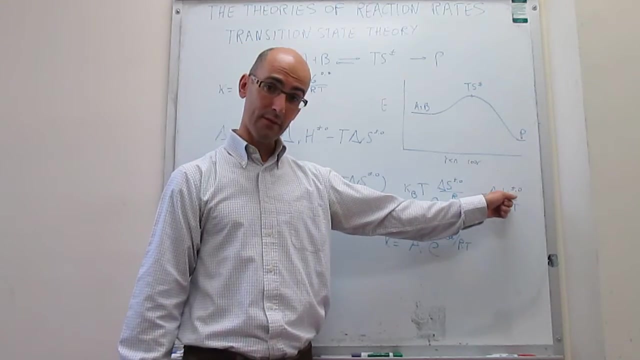 E, A over RT. okay, when we compare these two expressions, they actually look very similar. notice that in the Arrhenius theory you have an expression that depends on an energy divided over RT and here you have an exponential of an enthalpy divided over RT. okay, so this in principle gives you a relationship. 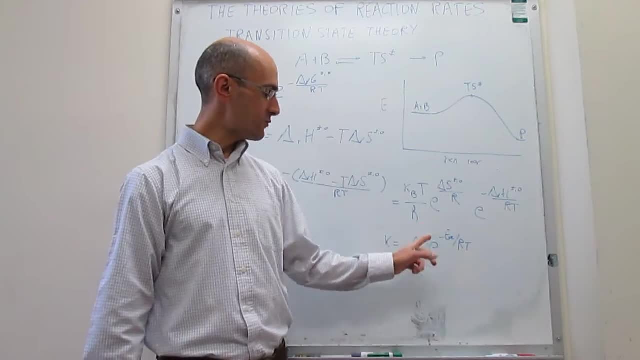 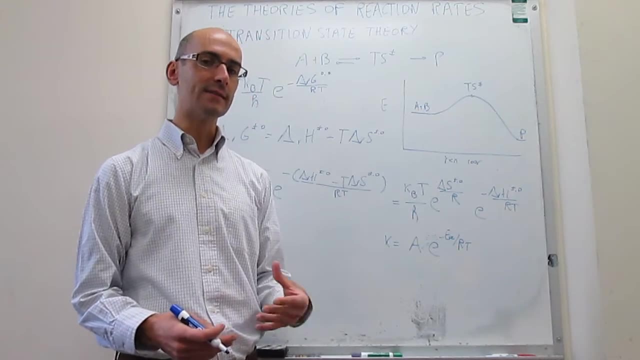 between delta H and the activation energy, and then the rest would be equal to the pre-exponential factor. okay, so it turns out that the activation energy and the enthalpy are actually not exactly the same thing. we know that internal energy and enthalpy are almost the same, but slightly different as a matter of fact. 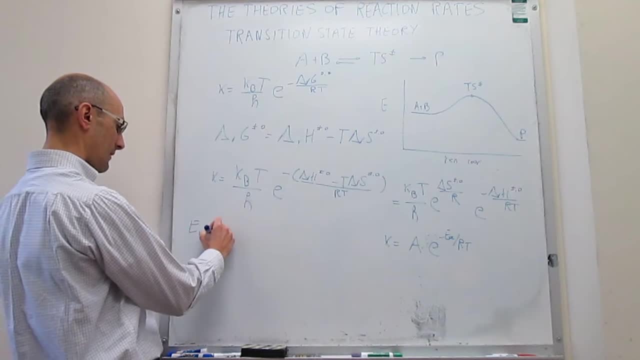 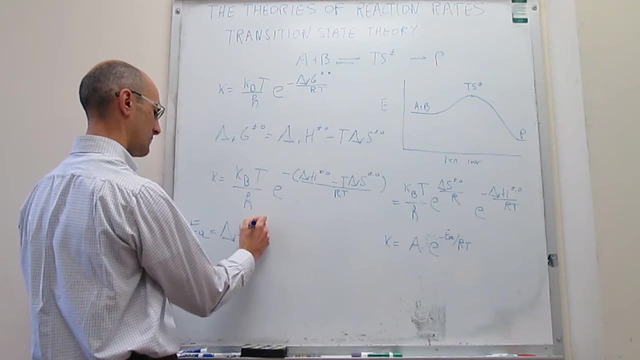 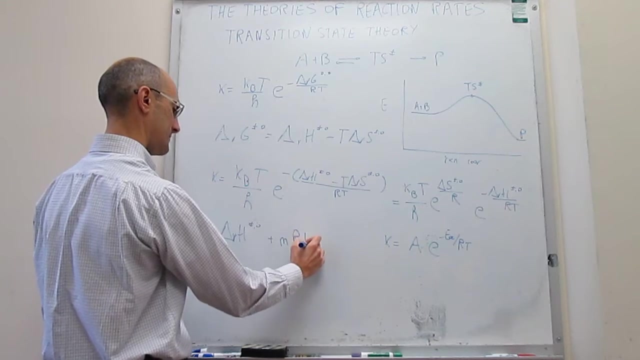 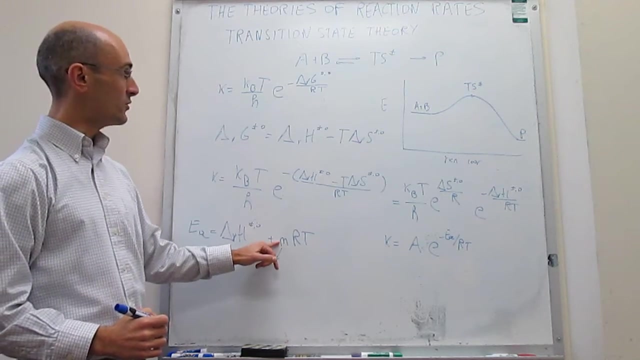 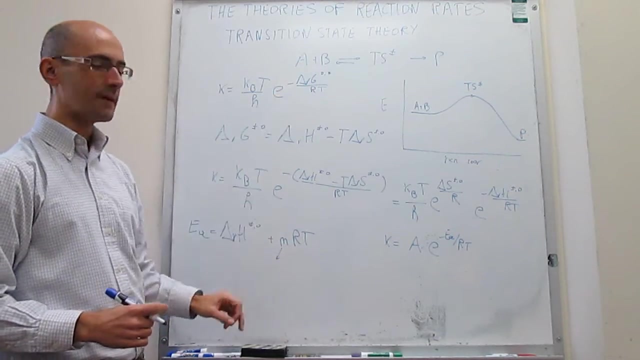 the true relationship between activation energy and the enthalpy of activation is this: R H activation plus M R T. okay, where this is simply the molecularity of the reaction. okay, so if this reaction is unimolecular, it only has one reagents, and this will be one. is this reaction is bimolecular, like in this case, then this: 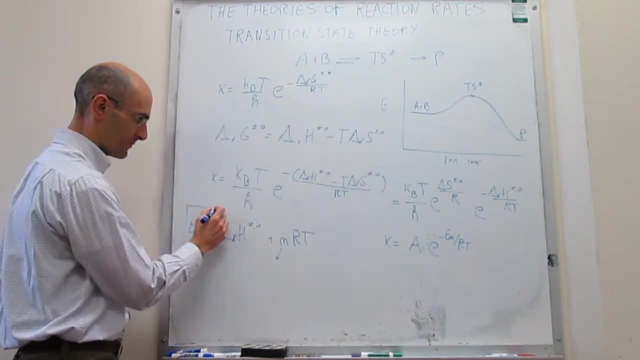 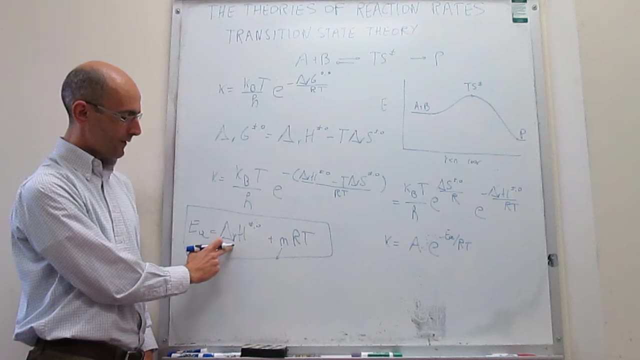 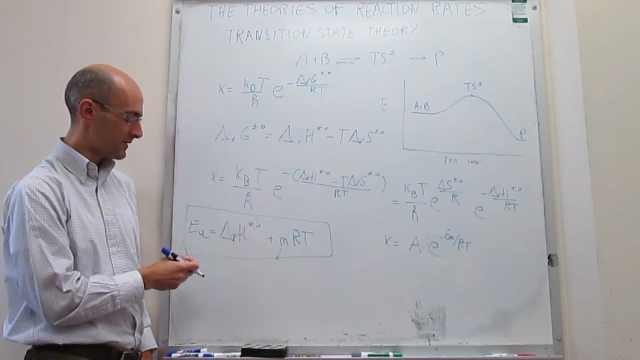 would be two. okay, so this is a very important expression, because a lot. it allows you to connect a parameter in the Arrhenius expression with something that comes from a transition state theory. they actually can. allows you to explain exactly what this activation energy is. well, the activation energy is simply the 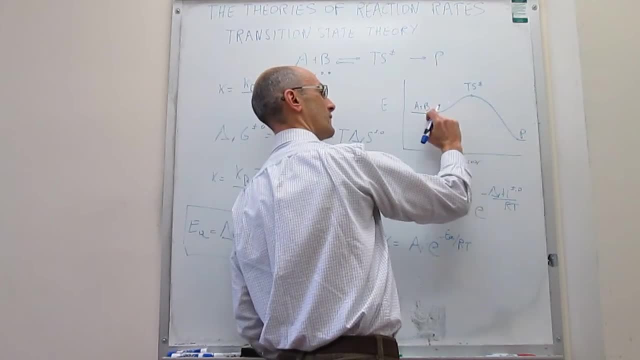 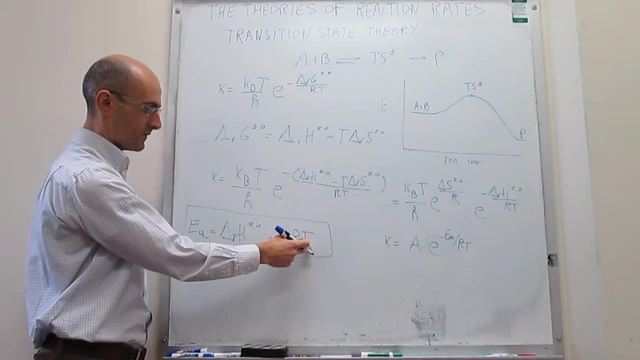 enthalpy, in the change in enthalpy going from the reaction from the Arrhenius to the transition state, plus a small correction, this is usually going to be very, very small Arrhenius temperature: okay, that depends on the temperature. okay, so again, this is the first, the first very clear explanation of what 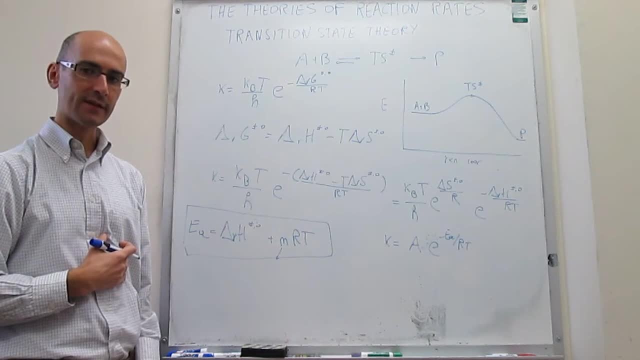 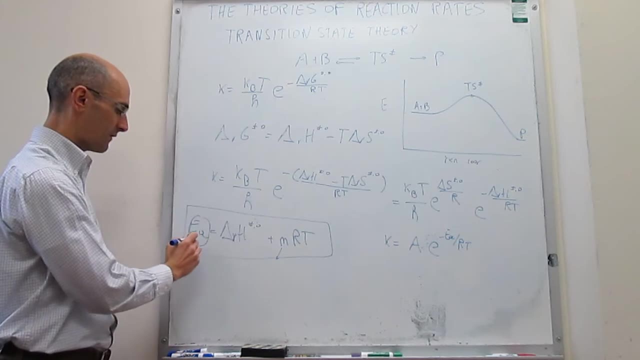 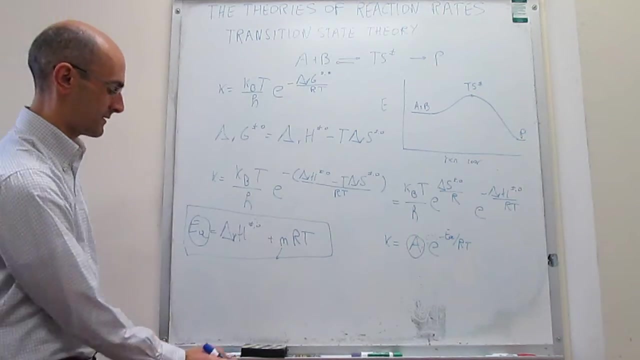 the dot para-parameter in the Arrhenius expression, activation energy, is okay. now the last thing that we can do, then, is incorporate this value of the activation energy into that expression, so that we can then find what the pre-exponential factor is. all right, so let's see if we can do that slowly here. so again, what? 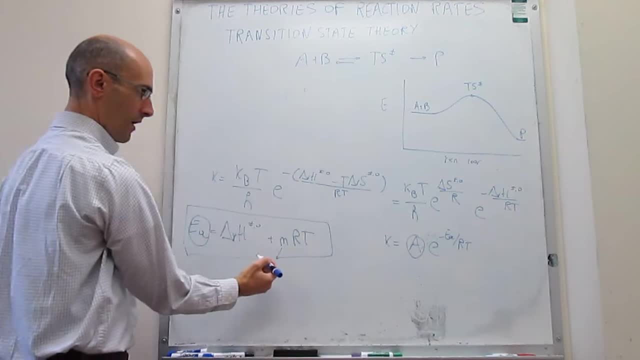 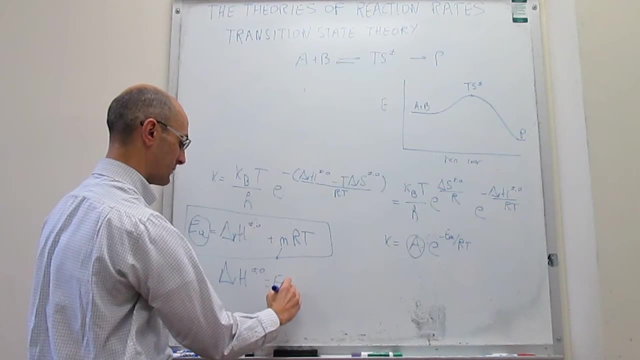 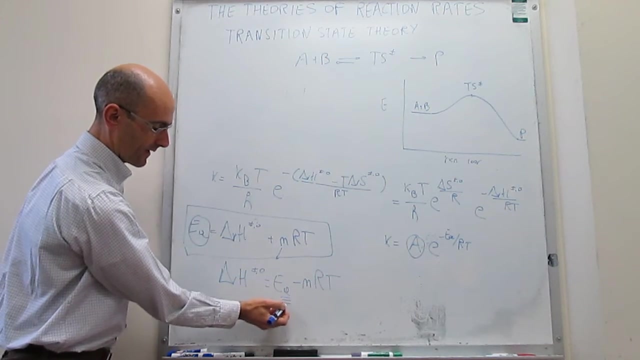 I'm going to do now is take this delta R H right here and then solve this expression for it. delta R H of activation is equal to the activation energy minus the MRT, and then this will allow me to plug in the activation energy into this expression. 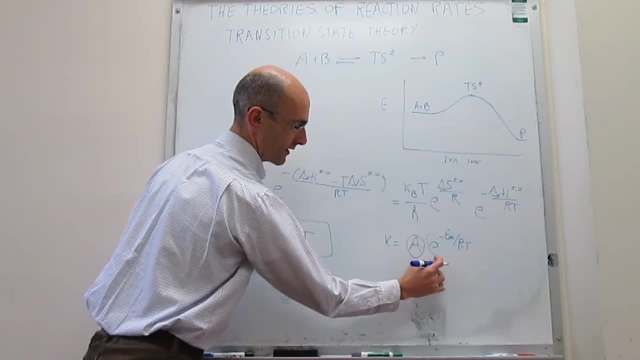 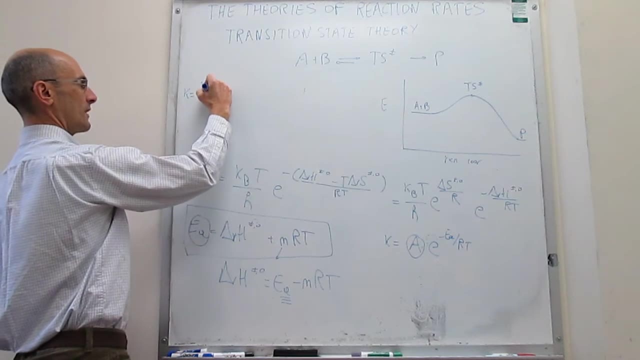 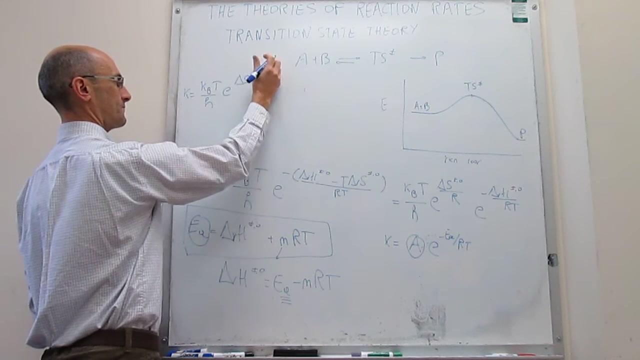 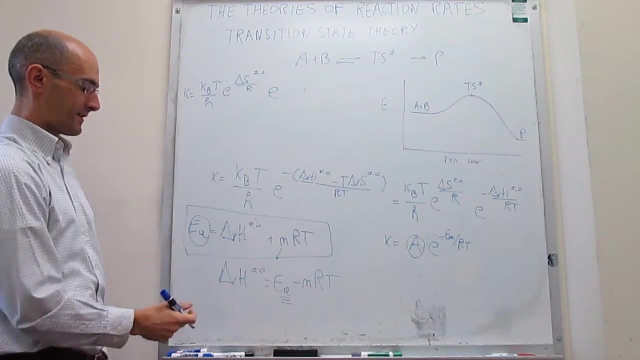 and then we will be able to establish very clearly what this pre-exponential factor is. all right, so let's see how we do that. this rate constant is going to be equal to K B, T over H, E of Delta S, of activation standard over R, and then we'll have E to the minus Delta H over RT. but then 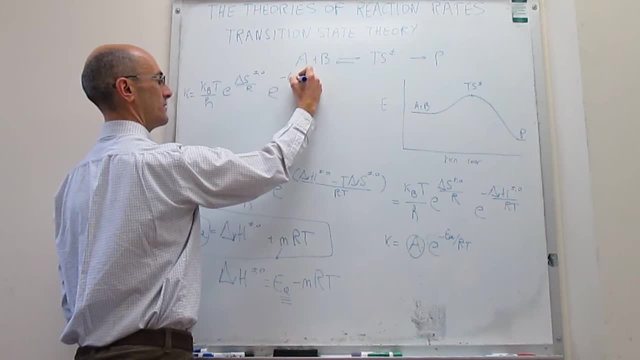 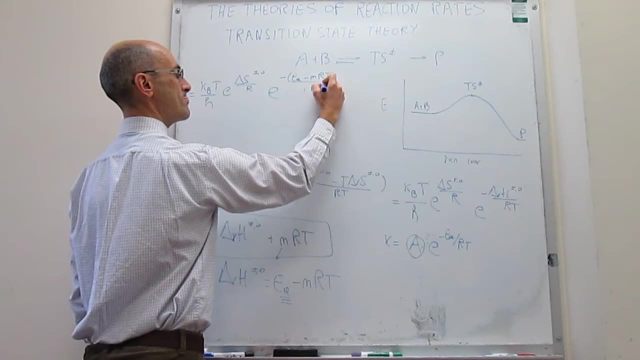 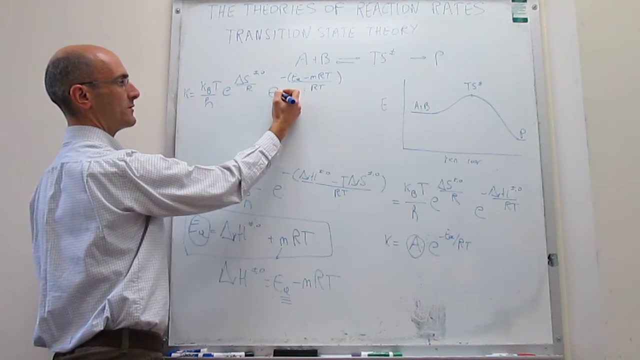 that's going to be all of these, minus the activation energy, minus MRT over RT. okay, and much as before, here we're going to have two terms. notice that this is going to one falling into the exponential of minus Ea over RT, multiplied by the exponential of. 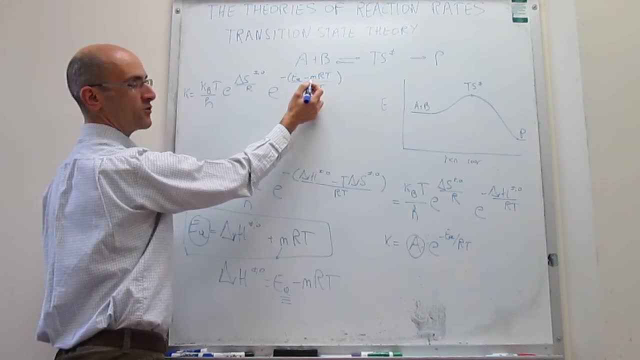 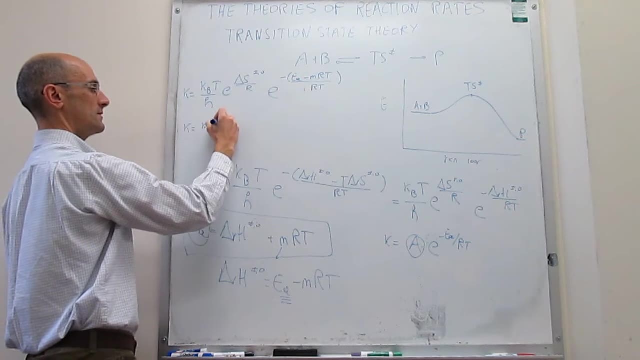 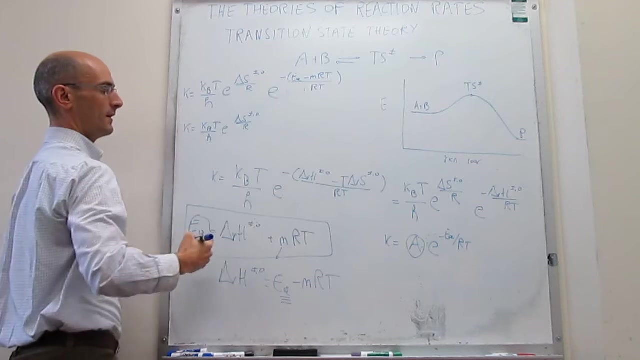 of plus MRT over RT, which is simply going to be e to the m. So our final expression is going to be like this: This would be t over h, e to the delta s of activation over r. And then we find that again here you'll have two terms. 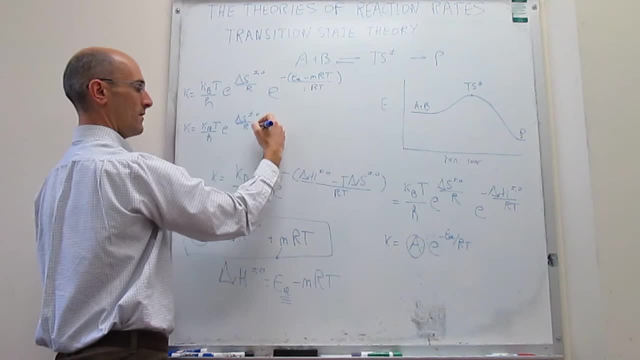 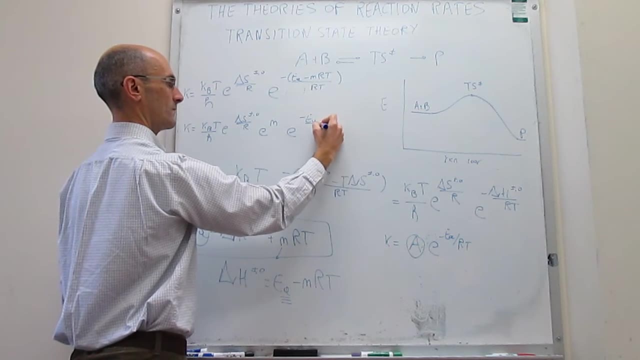 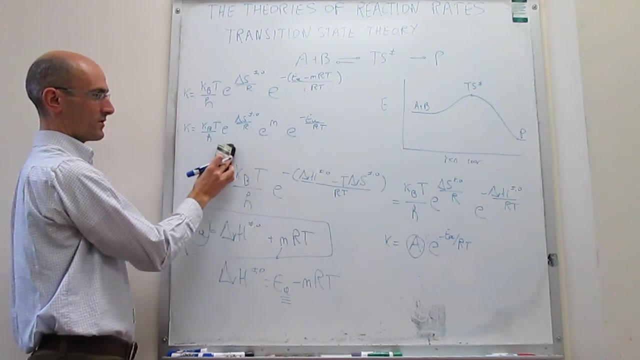 e to the minus ea over RT and e to the m. I'm going to write here e to the m first, And then the other term is this: And now this expression, which is a hybrid expression between Arrhenius and transition state theory. 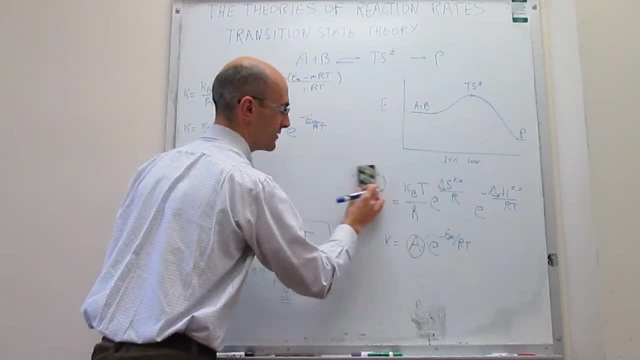 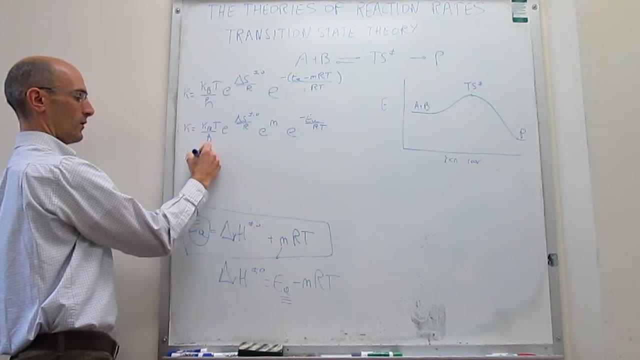 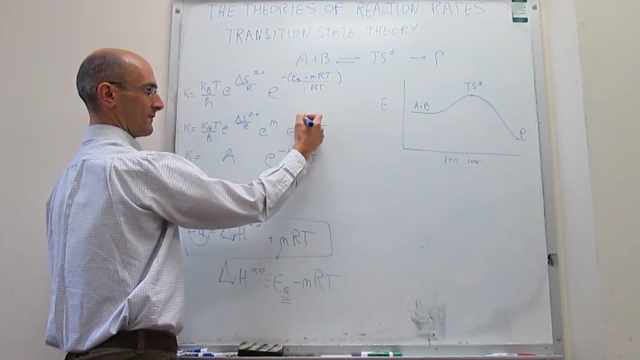 can be compared directly with the Arrhenius expression, so that we can actually see what the pre-exponential factor actually is. We'll write below here the Arrhenius expression. Notice that now, because we've been able to incorporate this activity, this activation energy, we have this term here. 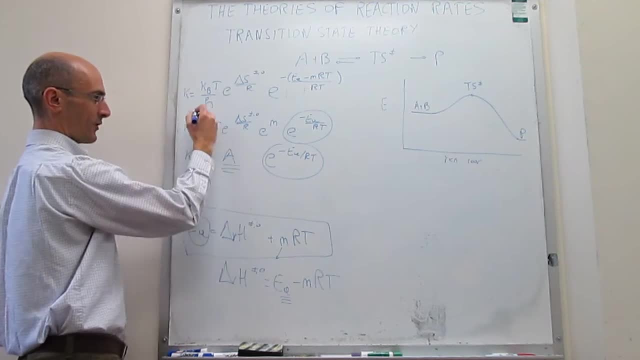 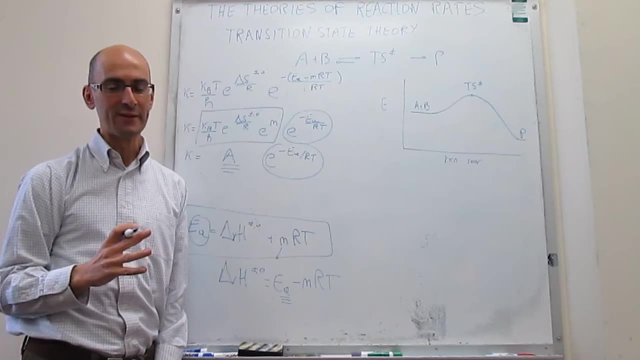 that is identical to the term there, And what that means is that the pre-exponential factor actually has to do with this value right here. So this is the first time that we actually get a glimpse from what that pre-exponential factor really means. 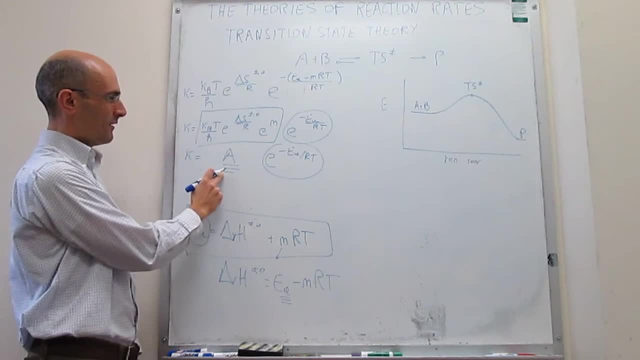 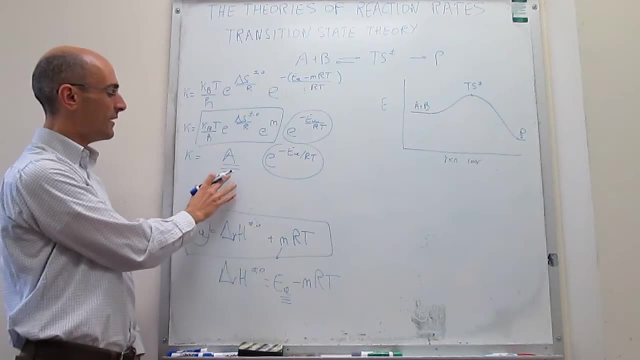 And the interesting aspect of this is that this pre-exponential factor, well, the first thing that happens is that it depends on temperature, And this is something that is not very obvious from the Arrhenius expression, where, at least when the temperature change is not 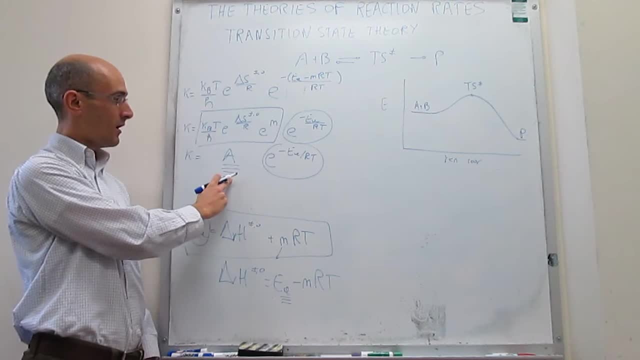 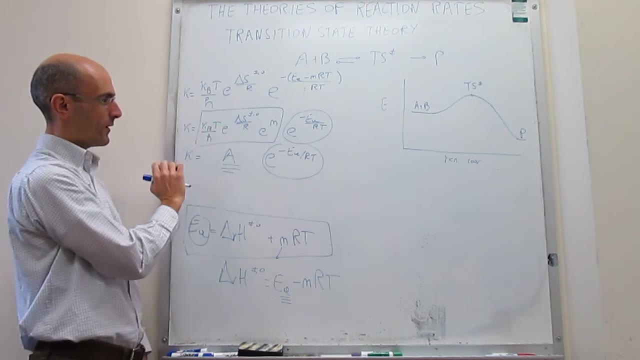 very large. we have assumed that this thing does not depend on temperature, But we see that when you actually take a detailed look at it, it does depend on temperature. as you have it right here. The second thing that is important about this pre-exponential factor: is it actually? 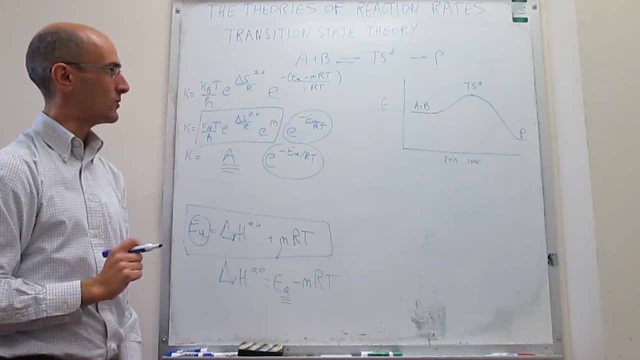 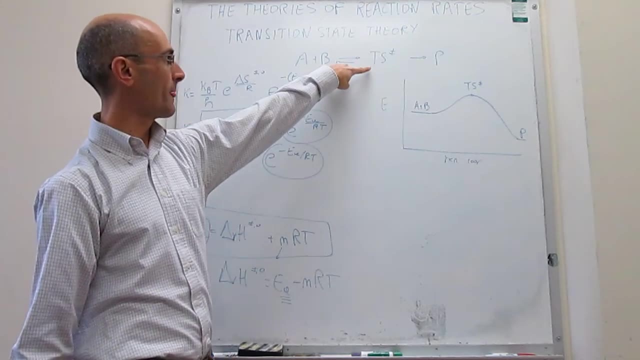 depends on the entropy of activation. And again, the entropy of activation is simply the change in entropy as you move from the reins to the transition state. For example, in this particular case where you have a biomolecular reaction, you will be able to see that this change in entropy 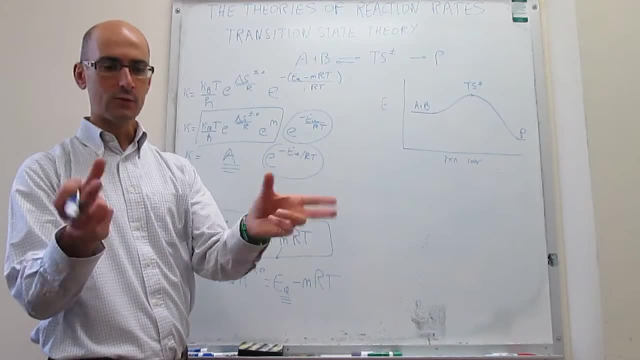 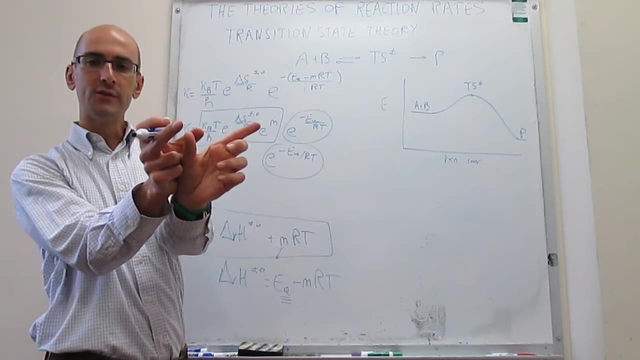 should have a negative value, because you're going from two species, the two reagents, A and B, which can have some entropy, to just one species in which those two are converging in space and bonds start to break and form. 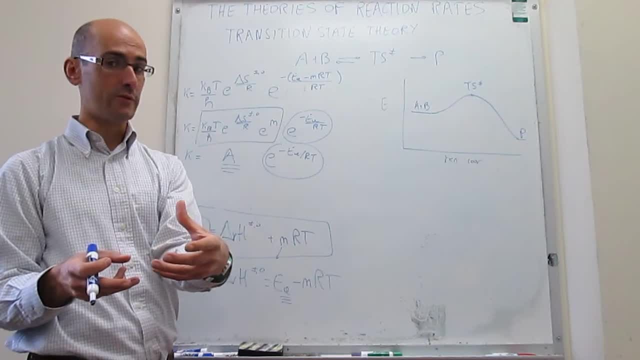 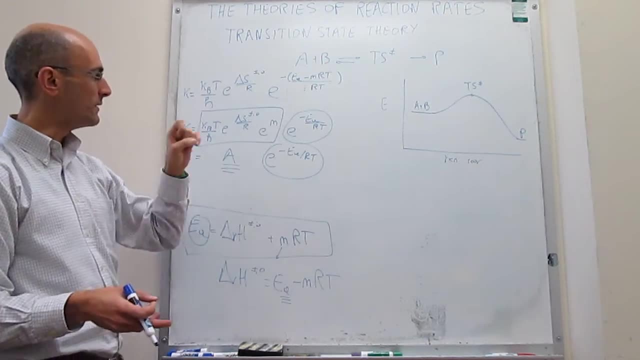 But you only have one species which is intrinsically more ordered, So you're losing this order as you go from the reins to the transition state In this biomolecular reaction. what that would mean is that this value here is negative, And again, this is something that 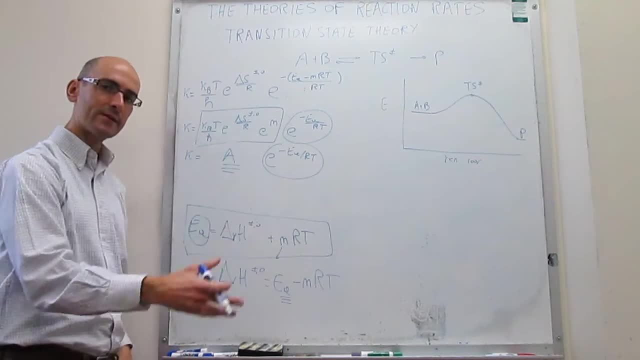 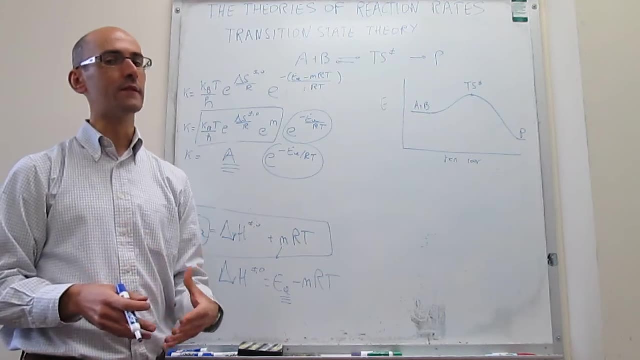 dictates what the pre-exponential factor is. All right. So, in summary, what we've done in this video is just take a thermodynamic view at how transition state theory and the useful thing of this is that now we actually have very tangible properties that 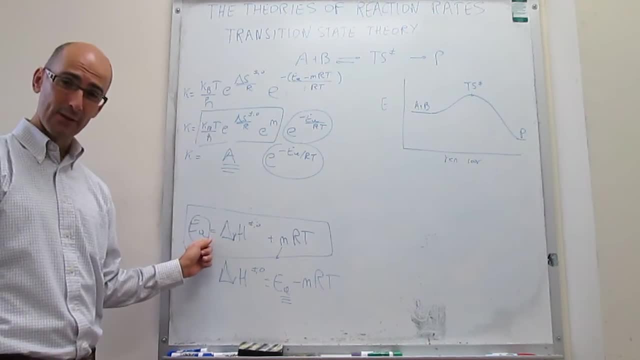 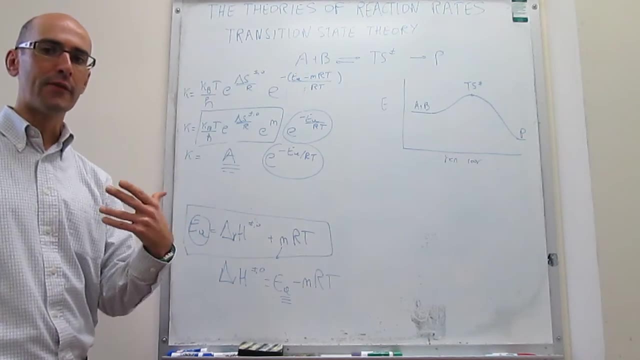 inform to us what the activation energy is- This is a value that appears in the Arrhenius theory- And then what the pre-exponential factor is, which is also part of the Arrhenius theory. OK, so again with thermodynamic arguments. 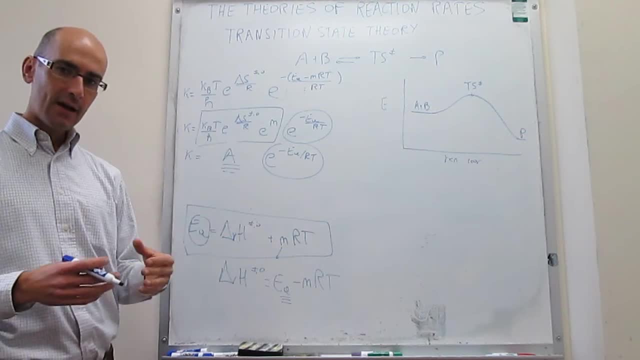 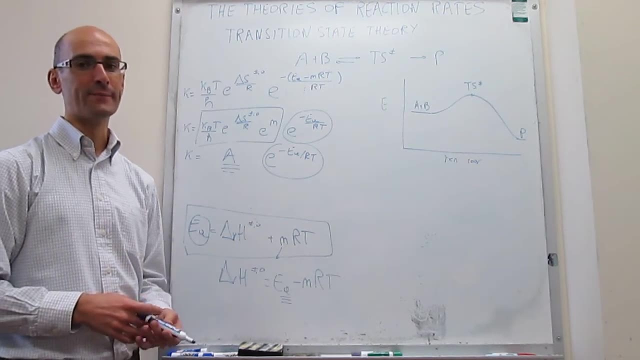 we're able to explain what each one of those two parameters are And in the homework problems you will actually get an opportunity to actually crunch some numbers and see what this value is really.